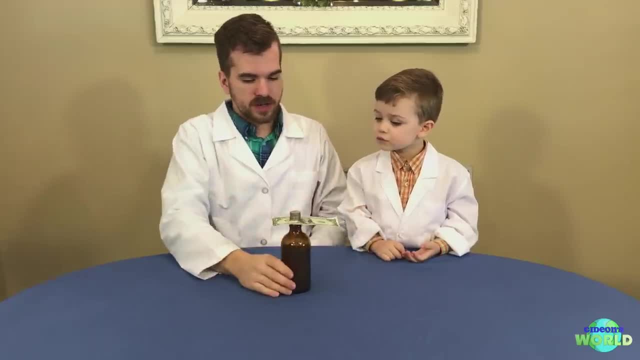 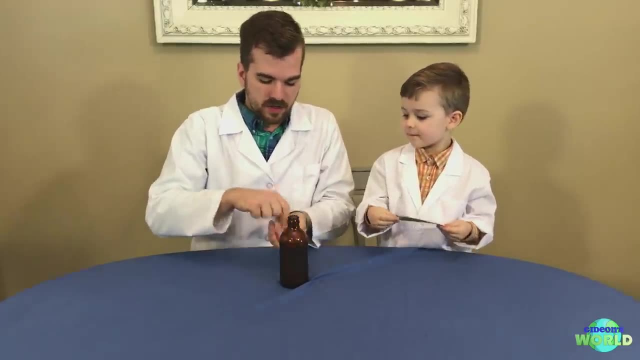 Normally, if you were to just grab this dollar bill and yank on it, try that The coins fall. Gideon was an outside force and grabbed the dollar bill, pulling on it, making the quarters fall. We're gonna try to create least amount of friction. 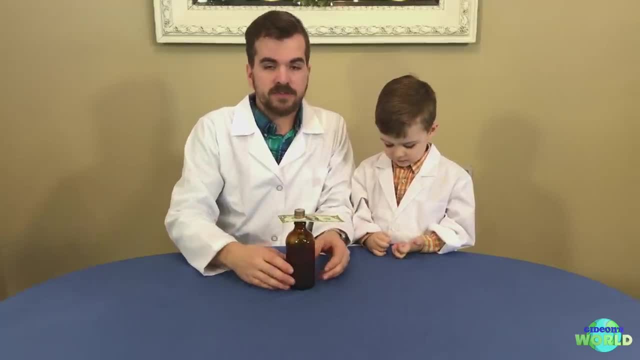 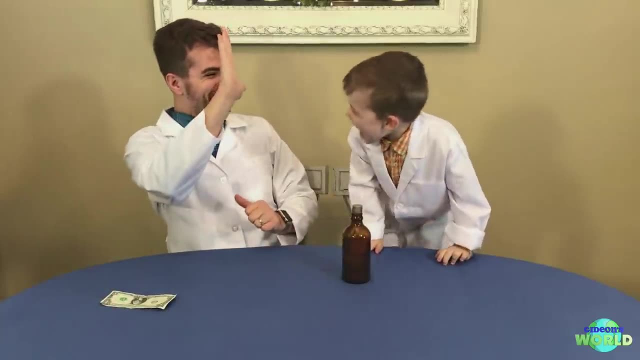 as possible and we're gonna pull on this dollar bill super fast. In fact, we're gonna karate chop it. Are we ready? Yep, One, two, three go. Oh, High five. dude, I got one point, We did it. 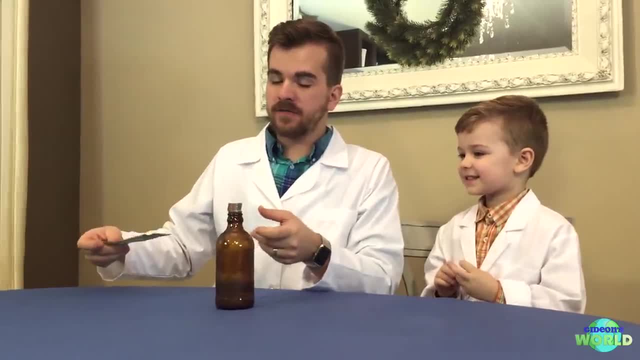 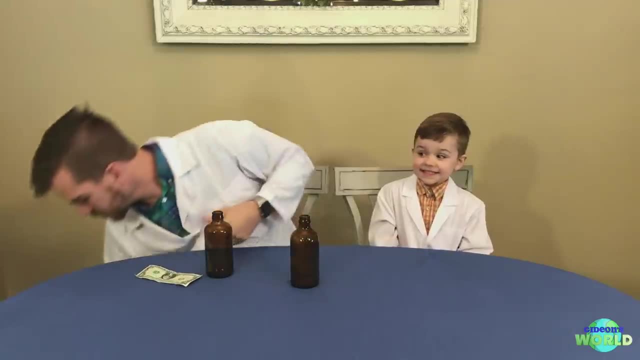 Basically, what happened was Gideon moved the dollar bill fast enough to where we didn't create hardly any friction, and that dollar was able to slide out from underneath the coins, leaving them in place. We're gonna up the ante a little bit. You ready, Yeah One. 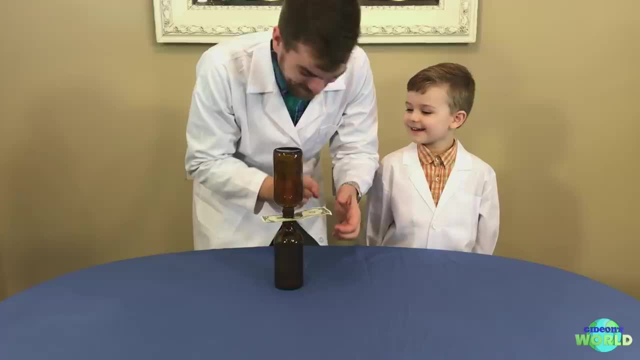 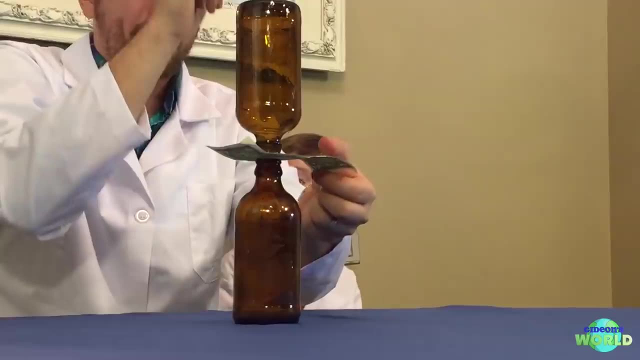 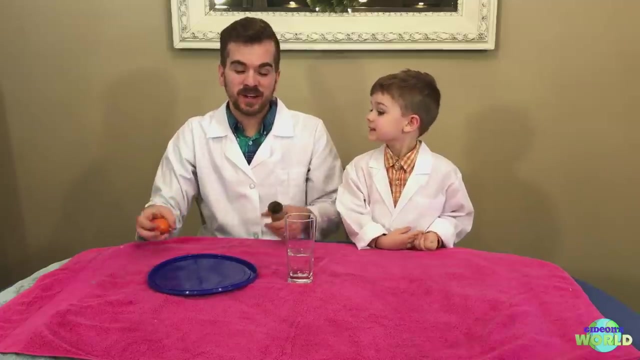 two, three. Are you ready? You're not ready. You ready? Yeah, Okay. Oh Yes, Almost feels good as a marker flip, Yeah, Okay. so this one is also about inertia. This one's a little bit cooler What we're gonna. 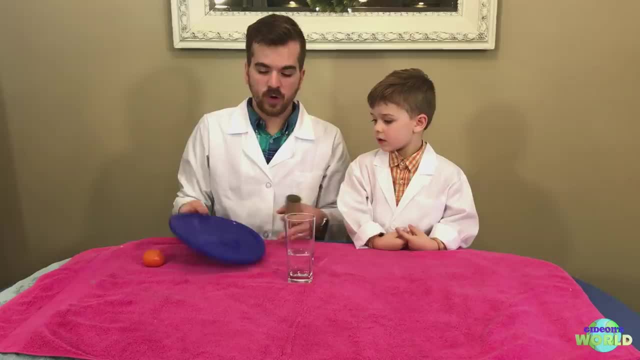 do is: all you need is a glass with a little bit of water in it, because it adds some weight. We're gonna put the lid on top. Then we're gonna take a little roll of toilet paper. You wanna line it up to where it's directly over top? 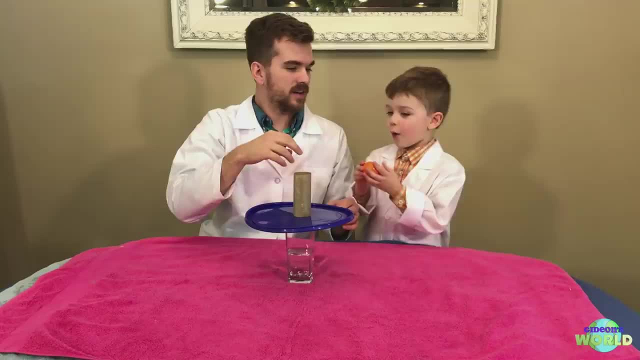 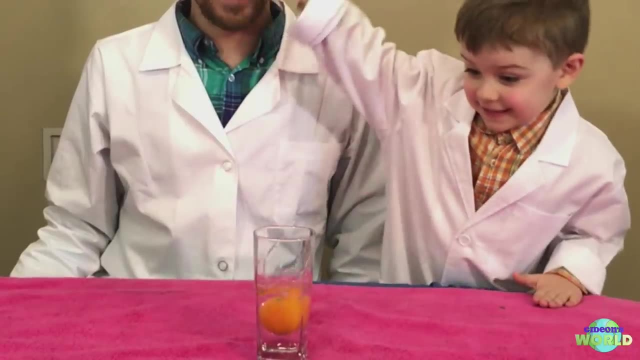 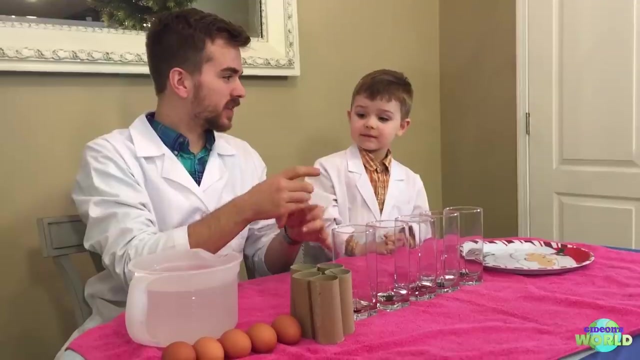 of the glass, like so, And you use an orange, But we're gonna use an orange. Okay, be real easy, easy. So you know how you did yours with the orange. Okay, just one by itself. Yes, and I hit it and it worked. 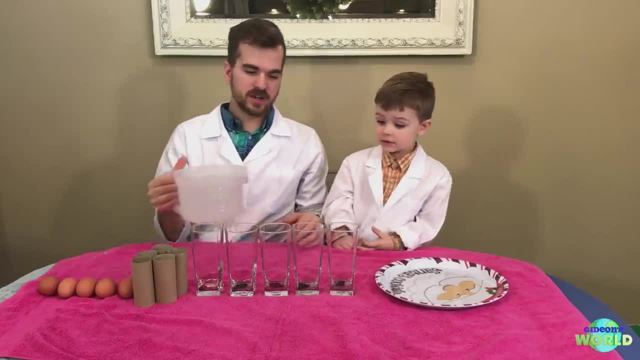 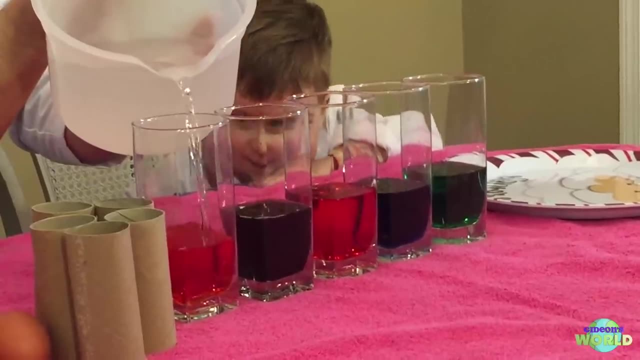 on the cup. Yeah, We're gonna up the ante. So we got five glasses here. We're gonna put some water in each one: Green, blue, red, black, another red. The color's not important. We just wanted to do colored water to be fun. 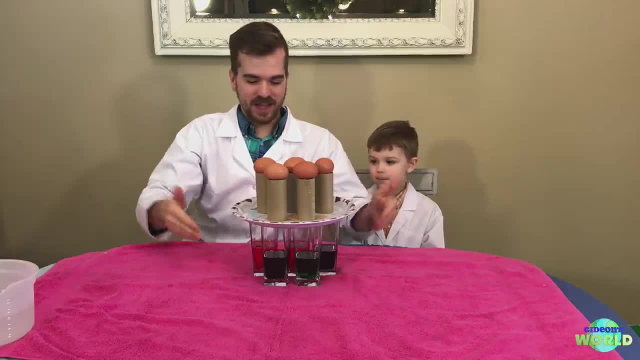 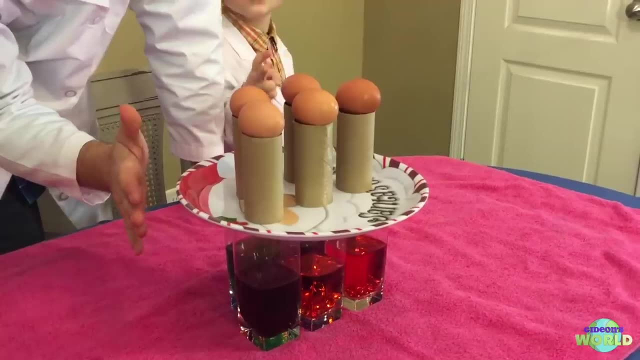 So we got five eggs on toilet paper rolls on the plate over five glasses. Daddy's gonna hit the plate and hopefully all five eggs drop in. Are we ready for this? Yes, You ready. One, two, three, Woo. 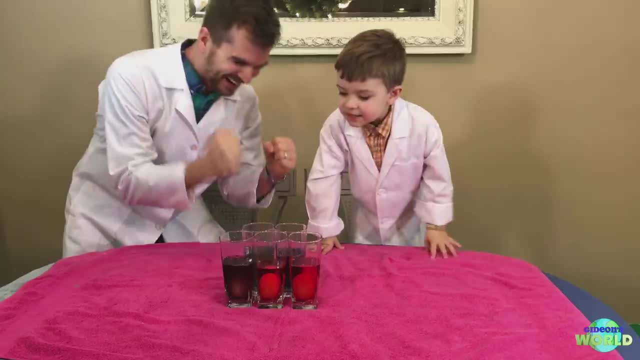 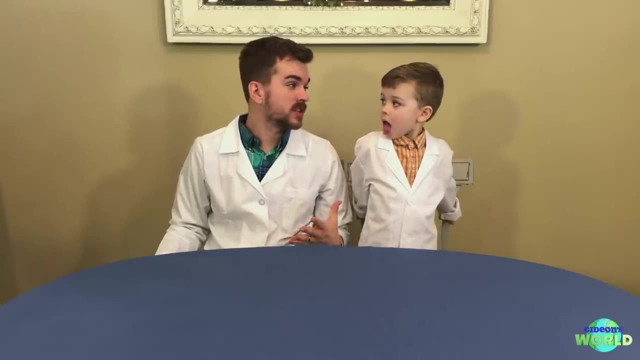 Woo, We did it. We got so many eggs Made it happen. Okay, Gideon. now this one is more about force We're gonna deal with. can you say centrifugal? Centrifugal, Pretty close And centripetal. 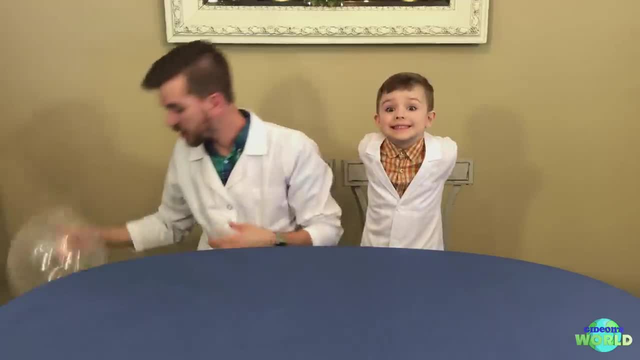 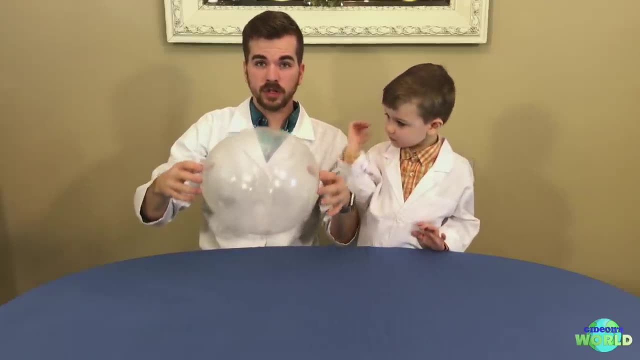 Centripetal, Centrifugal and centripetal force. So how we're going to demonstrate that is with a balloon with a penny inside. See, We're going to spin the balloon and as we spin the balloon we're going to create centrifugal force, which is 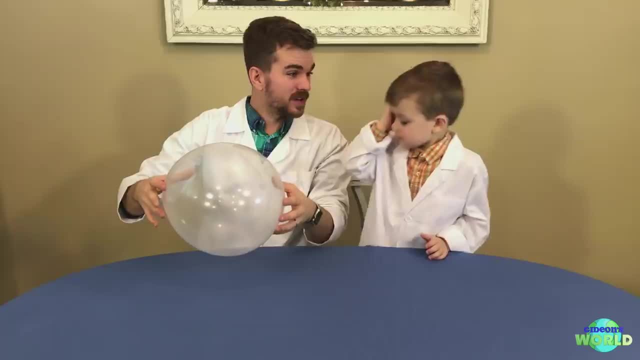 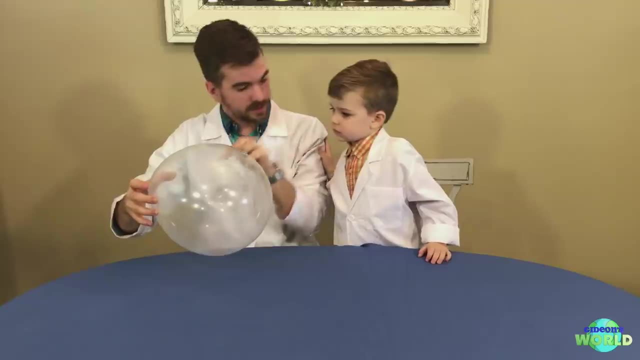 pushing the penny outward towards the outside of the balloon, But centripetal force is actually the layer of balloon which is holding the penny inside. Okay, Drawing it back towards the center. Are we ready? So all we gotta do is start spinning it. 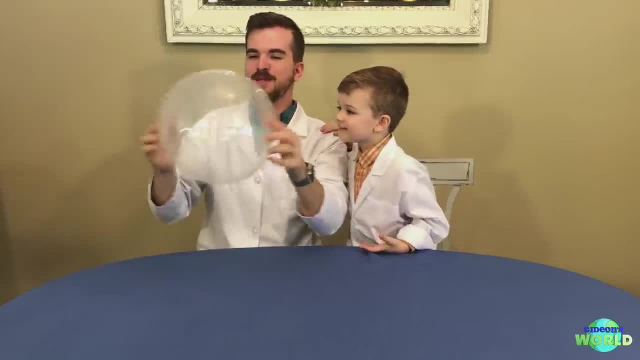 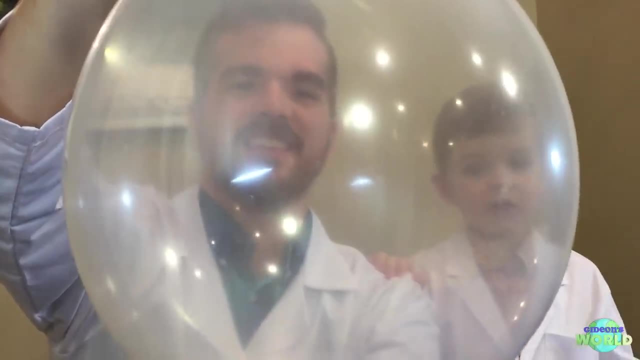 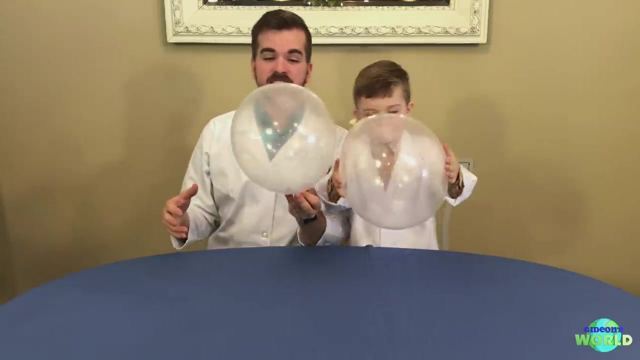 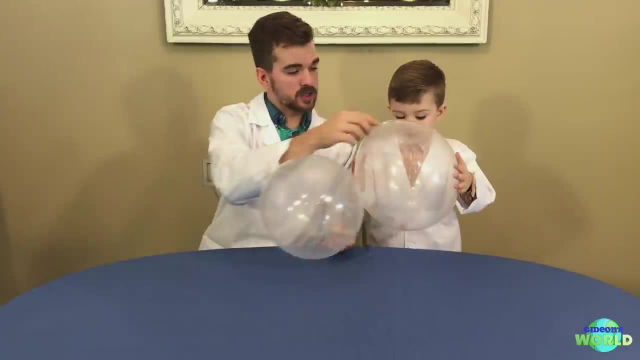 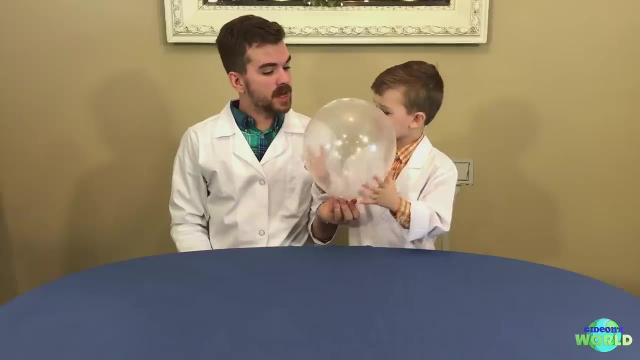 experiment. only, instead of a penny we got a hex nut. you wanna show them how the hex nut works? yeah, we put a hex nut in there. what it does is, as those sides hit the edge of the balloon, it makes noise, it vibrates, so get it spinning. 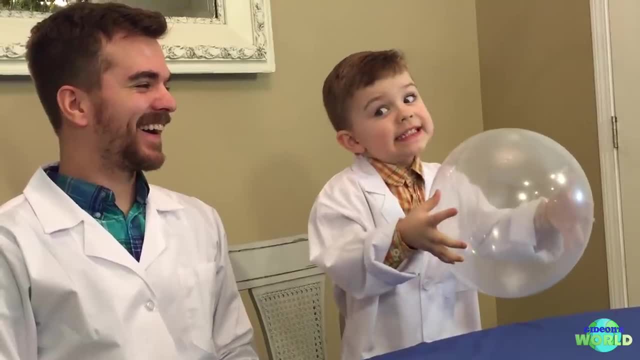 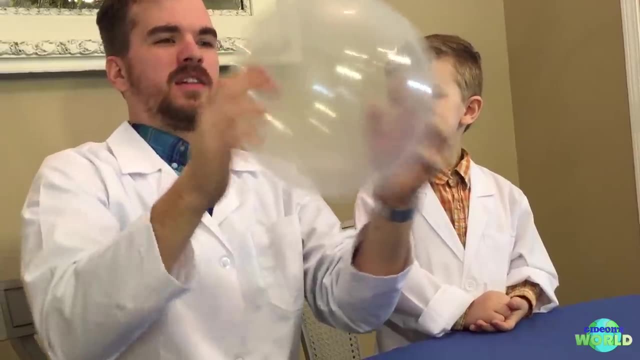 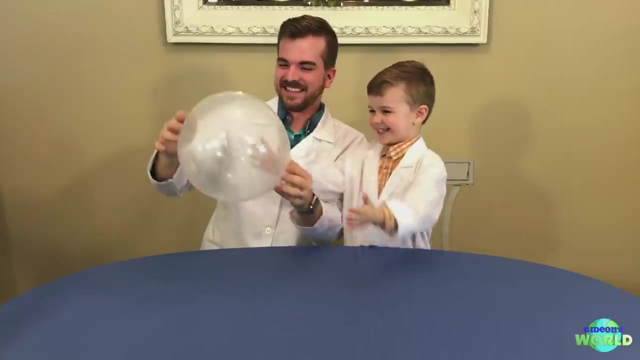 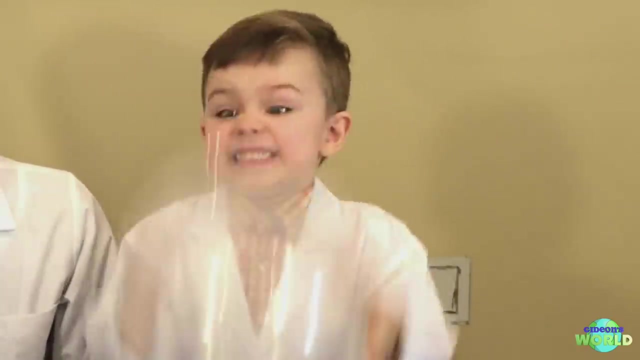 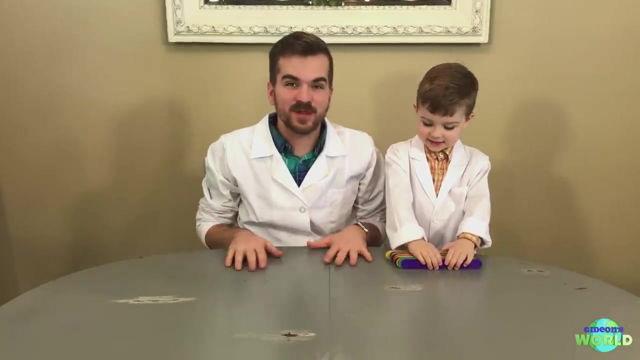 if you got a lot of these going at once, it probably make a lot of noise. see a lot. I can get it. it's fun, isn't it okay? getting you ready for our next experience experiment? yeah, okay, this one's more about energy. this is more like potential. 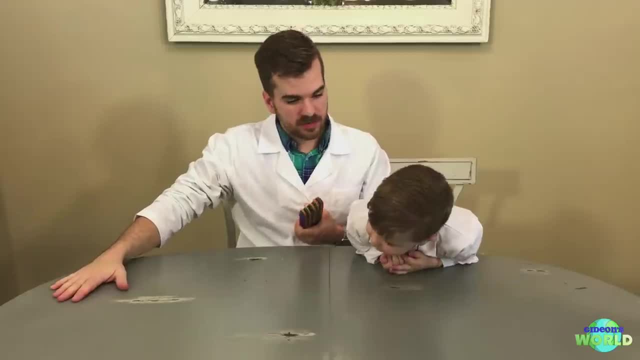 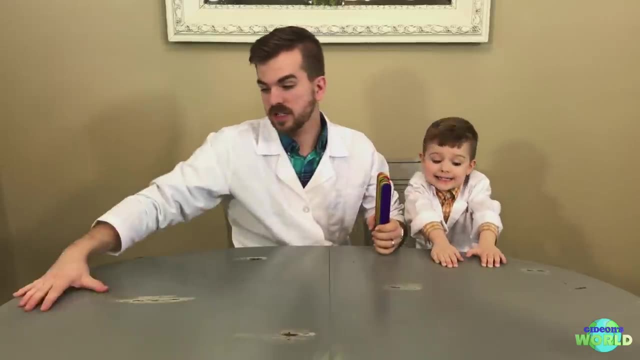 energy and kinetic energy, and we're gonna build it's called a popsicle stick bomb. we're going to weave them across and, as you weave them a certain way under and over each other, and building that potential energy, once it gets to the end, you create a trigger. we're gonna release it and it's gonna create. 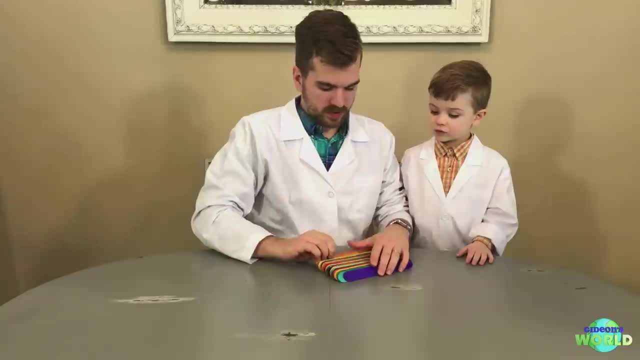 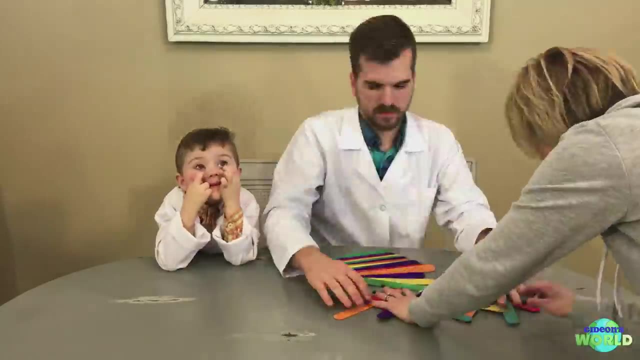 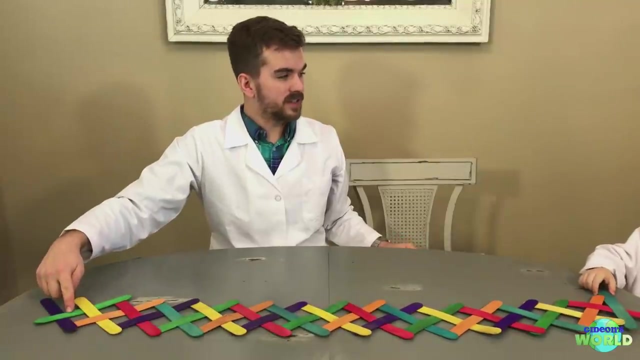 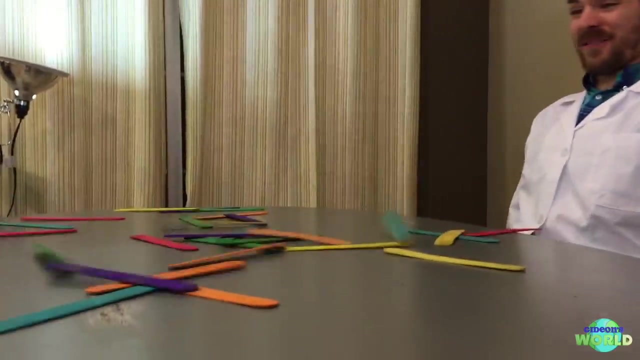 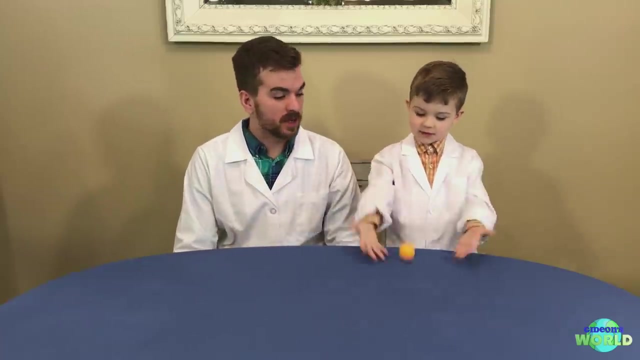 kinetic energy and it's gonna go boom and it's gonna blow all the way across the table. you ready? let's start red and orange. this is about Bernoulli's principle. he was a guy from a long time ago who discovered stuff about air pressure. okay, so we're balancing between low pressure. 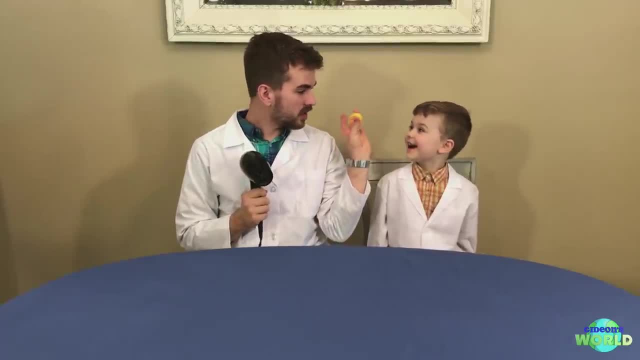 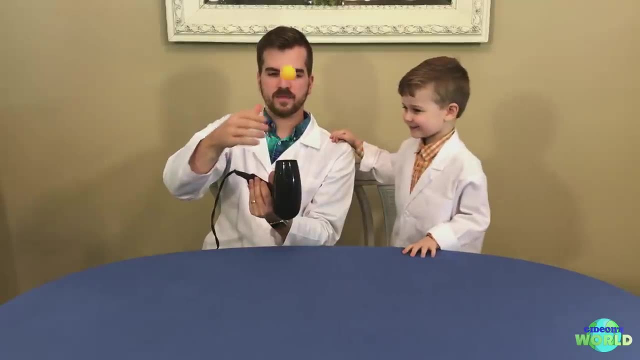 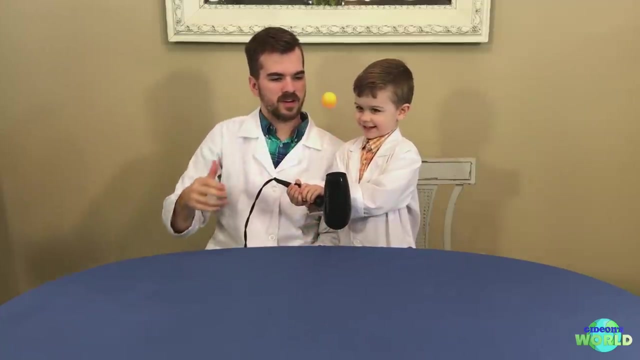 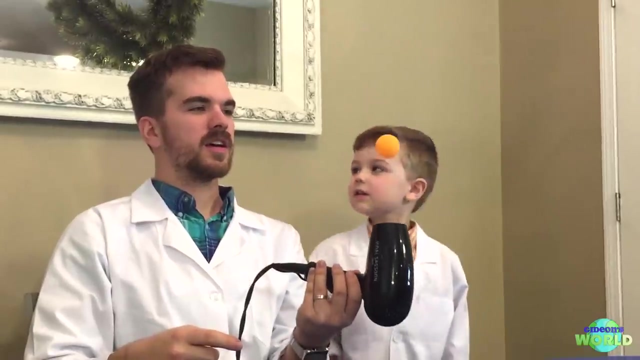 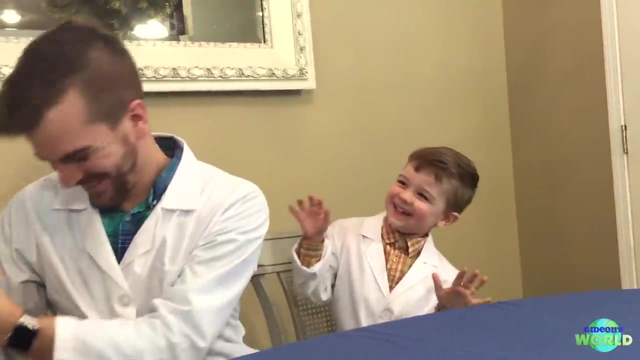 and high pressure. okay, we're gonna take his hairdryer. do you think we can make this float? yeah, it's almost like magic. let me try it like magic, but it's not. it's science. ready, set, go, are you ready? oh, we're gonna try this again, only with a. 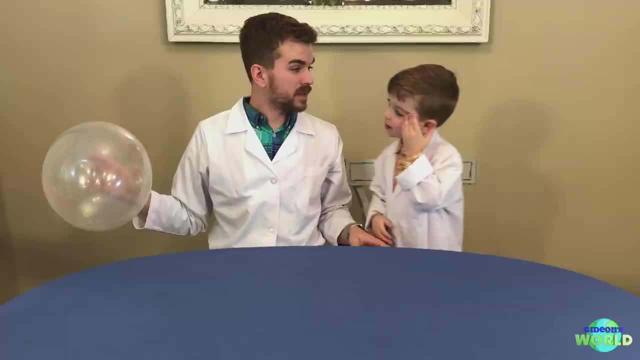 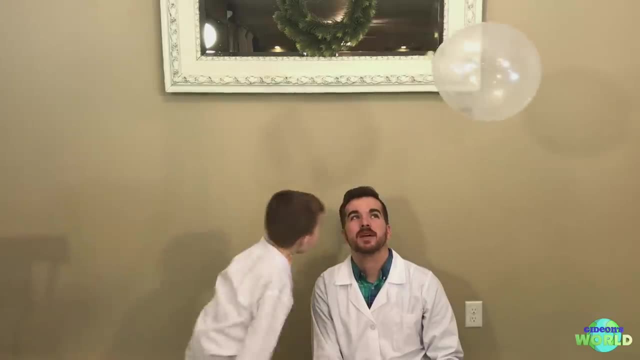 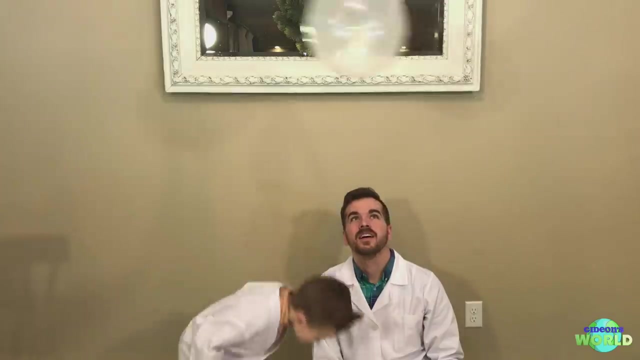 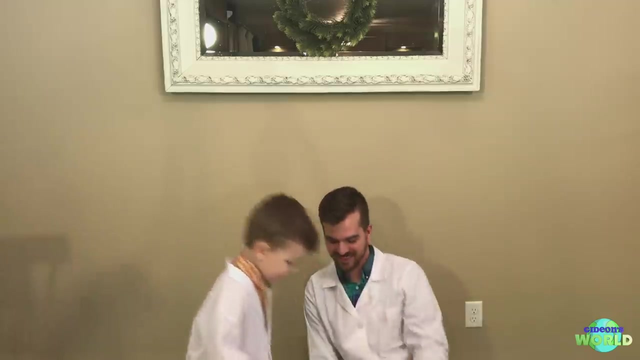 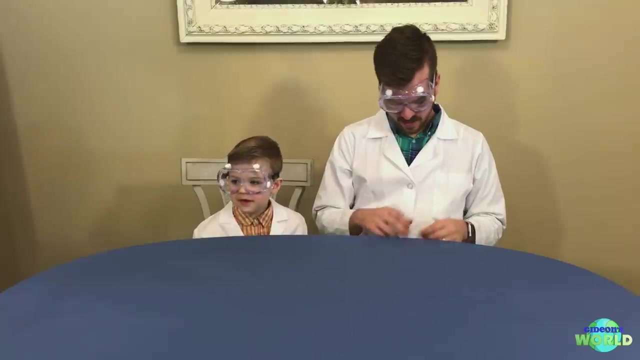 very nice, complicated, determined brain. We're gonna up up the. we're gonna up the airflow. okay, So check this out. This is another example of Bernoulli's principle: Where we're gonna Do is they're gonna take this toilet paper and watch the daddy blows across the top of it. 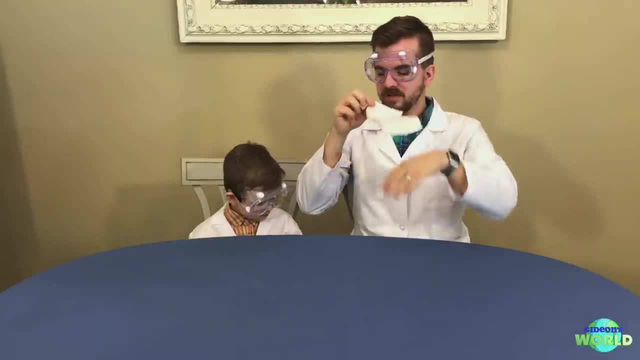 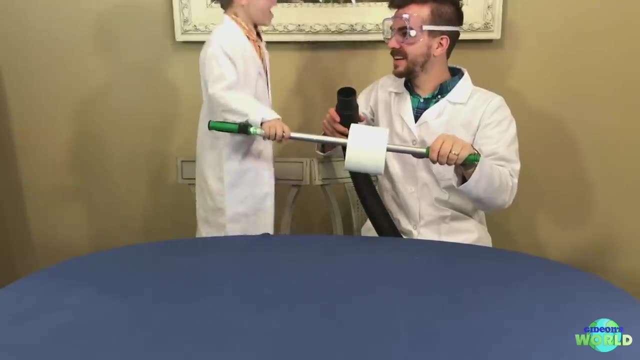 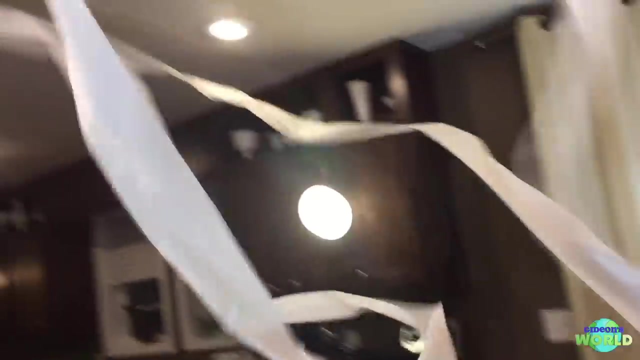 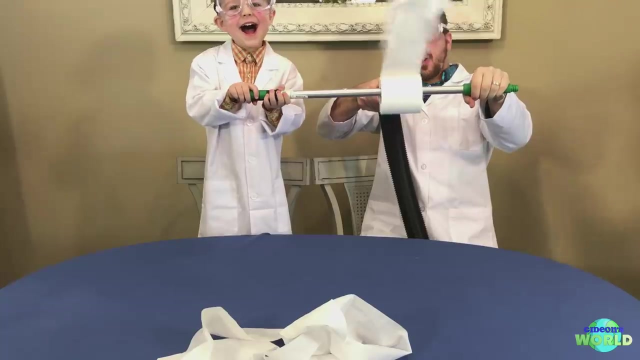 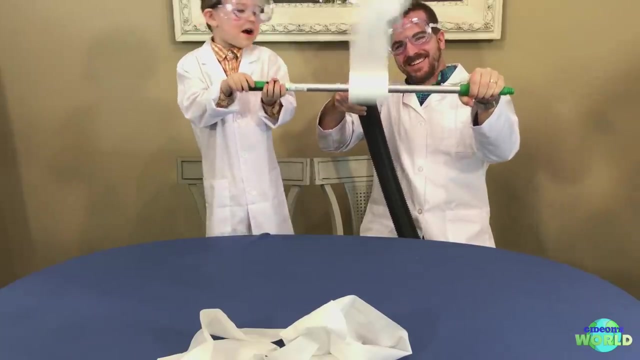 I'm blowing air across the top, but it's actually causing the bottom of it to lift up, and that's what we're gonna do. Are you ready for this? Yeah, That was awesome. Let's do that again. High five Guys, it's time for the balloon rocket. 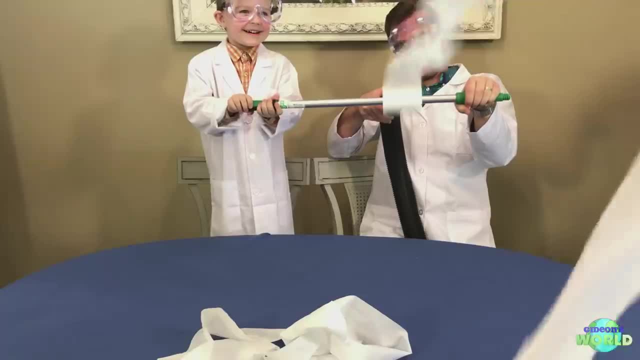 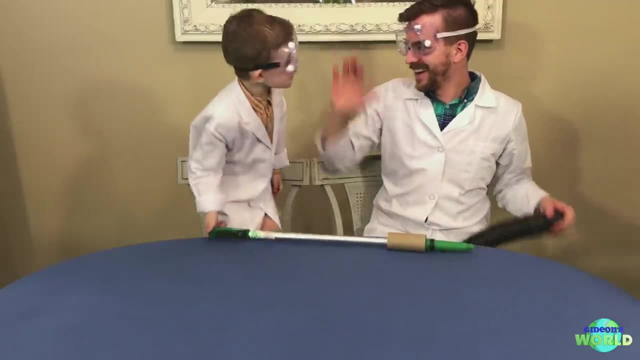 The balloon rocket. Let's have mommy come with us. come on, You gotta come over here Really fast. So we got a bunch of strings here And we're gonna tie it up, And then we're gonna tie it up, And then we're gonna tie it up. 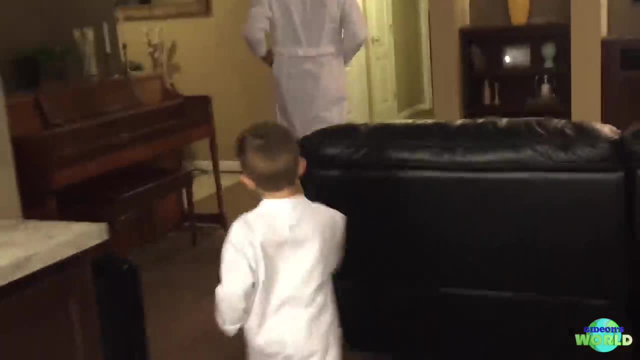 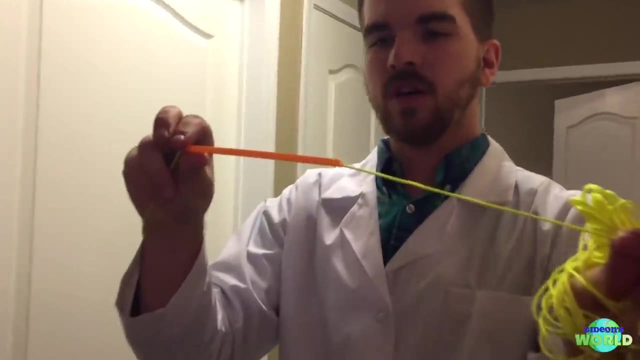 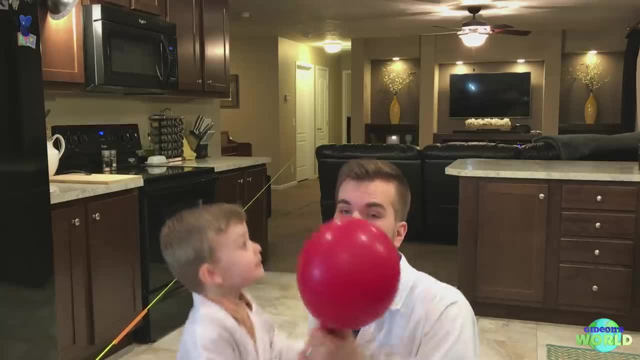 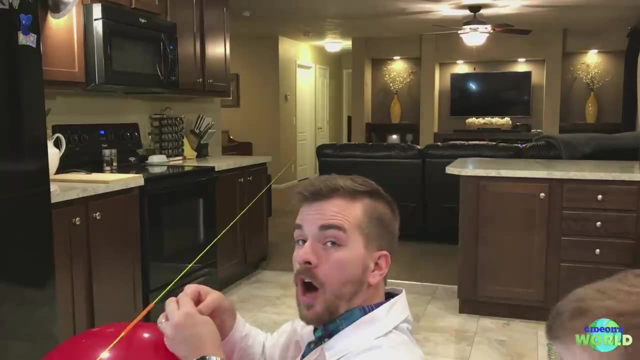 I took a piece of straw, cut the piece of straw, Put it on the string. okay, We're gonna try a big balloon first. This one gets really big, Really big. Stop it. Okay, now we're gonna take tape. Okay, now we're gonna take tape. 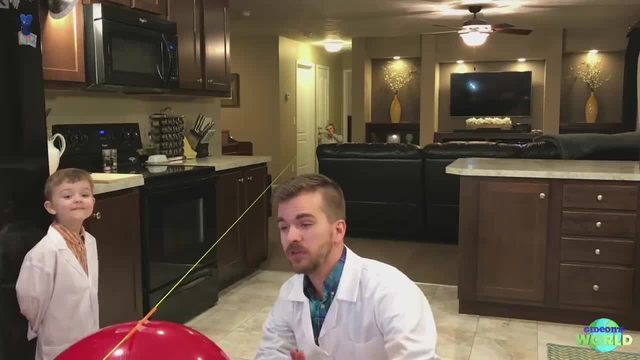 We're gonna try this with a big round balloon first. Now what we've done is we've filled this big balloon up With a bunch of pressure- okay, so air pressure With a bunch of pressure- okay, so air pressure Is really high in there, so there's particles that are just bouncing up and down. 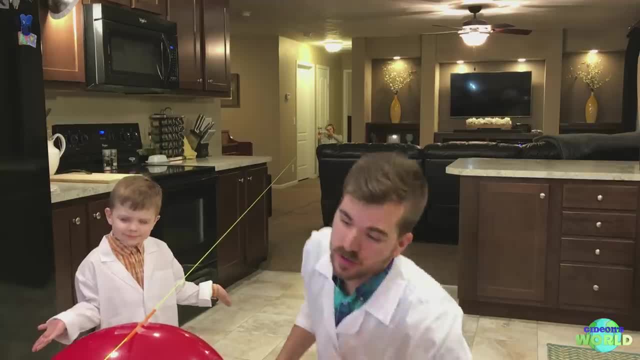 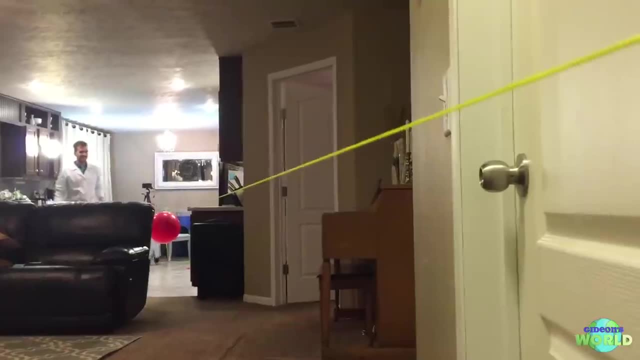 bouncing around like crazy, dying to escape. So what we're gonna do is we got a clothespin on the end, We're gonna let it out, Pressure's gonna release and it's gonna send the balloon flying. that way. There it goes. 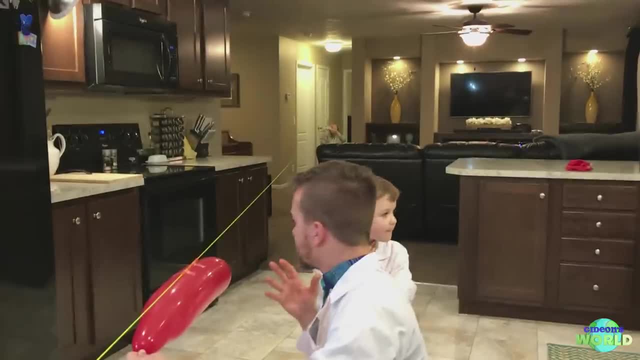 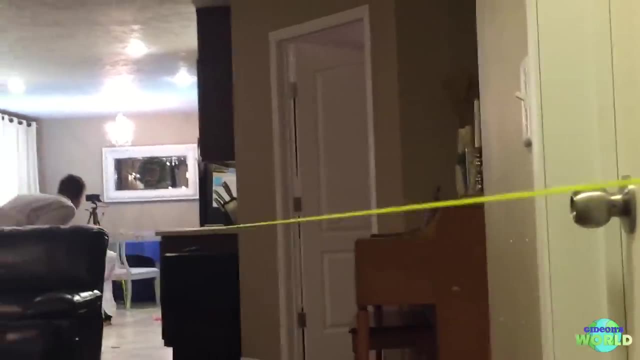 Not bad. All right, now we got a cylinder-shaped balloon. We're gonna test to see if this one goes faster. Are we ready? Yeah, Mommy, you ready Ready. One, two, three. Whoa, Did you see how fast that was? 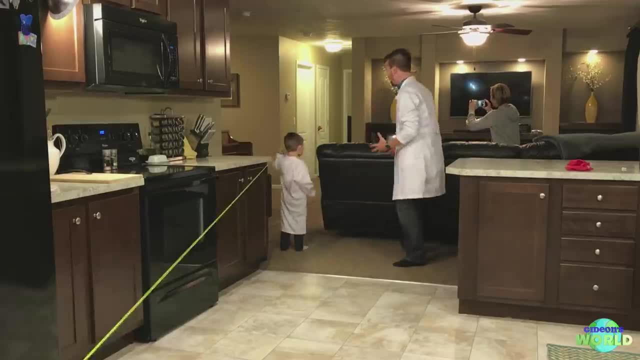 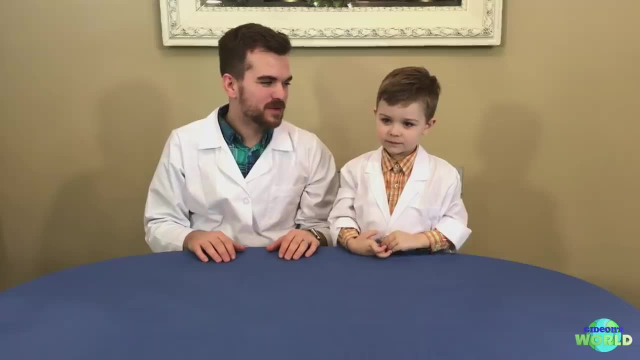 Three, two, one go. Whoa, That is a little bit cool. Thank you for watching Giga Go to Science. We did force-in-motion experiments, which was really fun. We don't just do science videos, we do gaming videos. 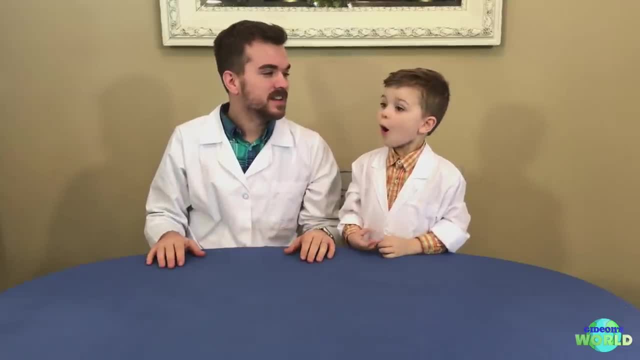 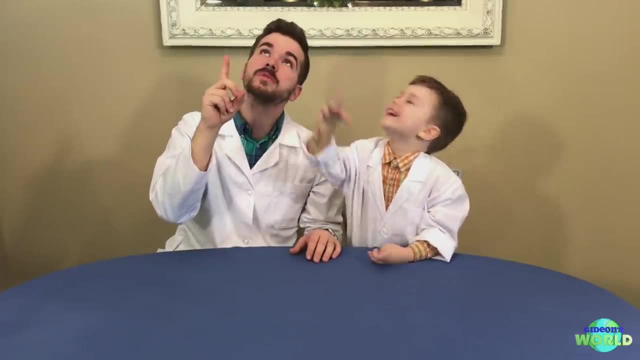 We do videos about toys, unboxing and all kinds of stuff. Oh, and the giveaway: It's up there. can you see it? It's up there. It's about our giveaway video. We're doing a 100-subscriber giveaway video. 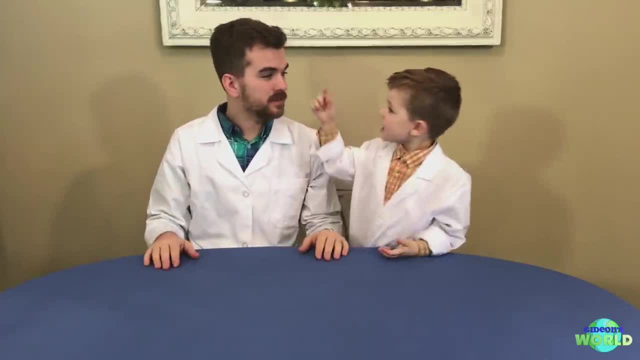 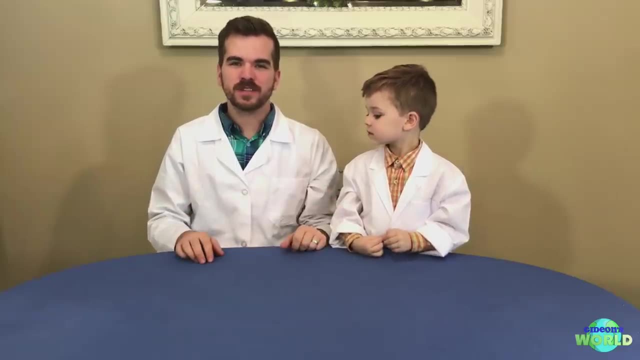 so check that out. Enter the contest. You can win a $25 Amazon gift card. And on Facebook: Yeah, we're on Facebook. We always have a link to our Facebook page in the description. It's facebookcom forward slash Gideon's World. 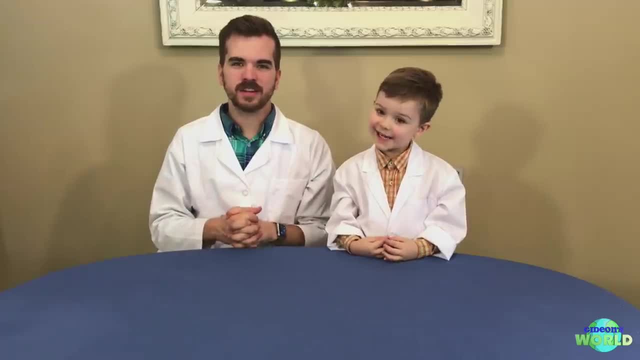 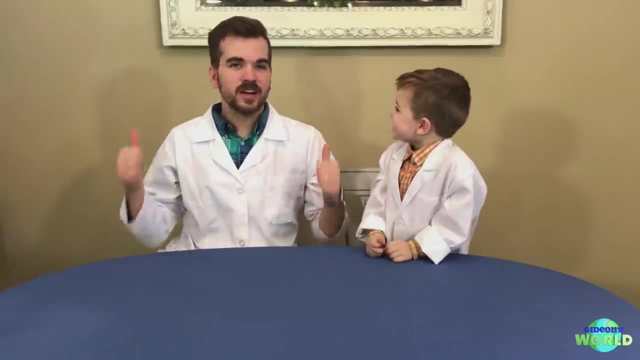 It keeps up with all the cool stuff that we're doing. We also do behind-the-scenes pictures and stuff like that, So be sure to check us out, like us and follow us there. Click this button down and please subscribe. Like this video. leave comments if you got them. 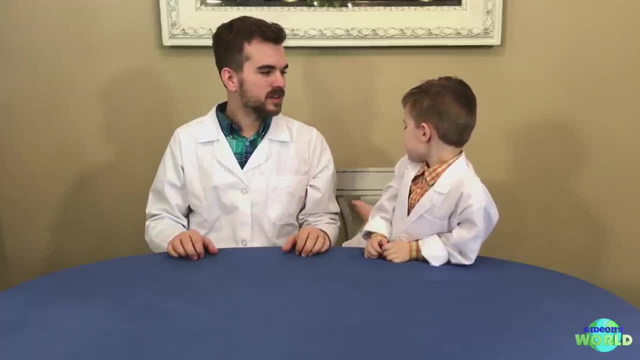 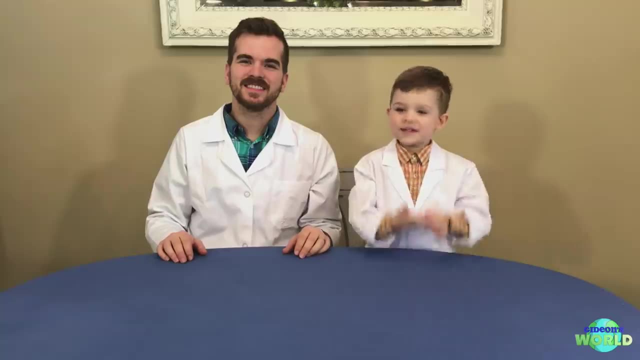 any suggestions for upcoming videos? We do new videos every week, don't we? Yeah, and every single week, And who knows what we're gonna do next? Thank you for watching Gideon's World of Science. Yeah, we'll see you, guys next time.